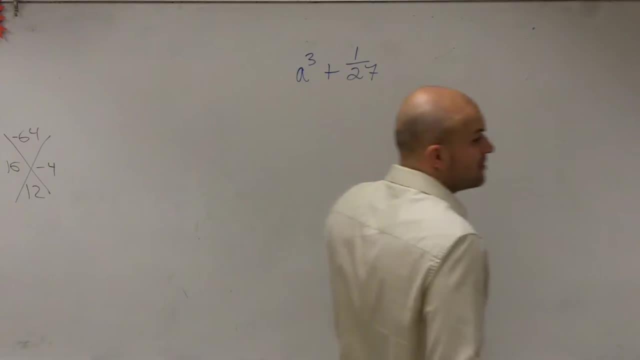 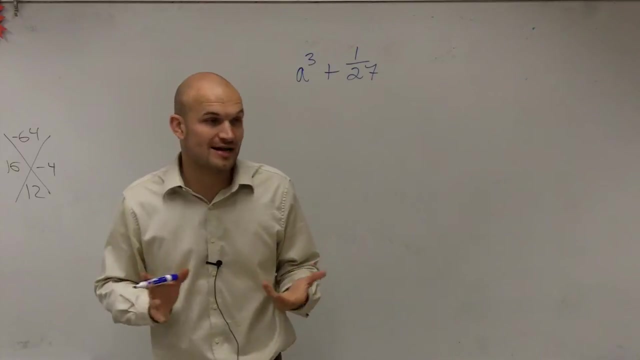 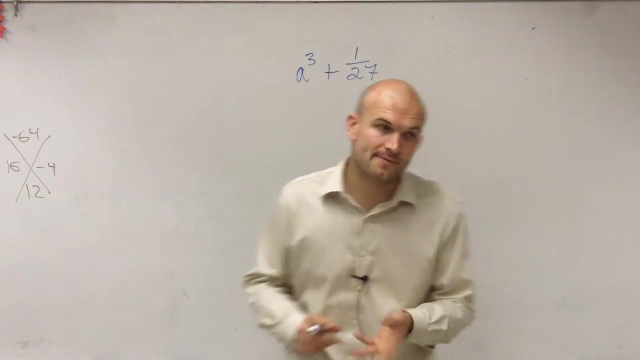 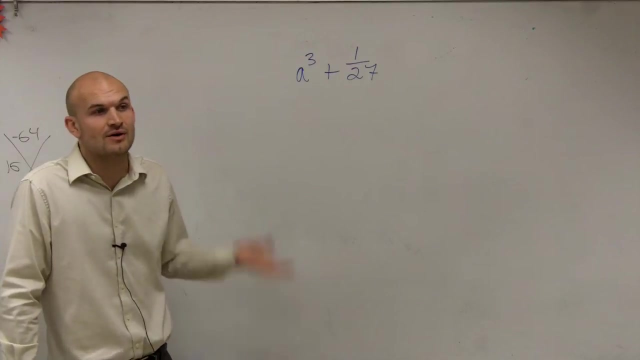 All right. so what I have is the sum of two cubes. I have 8 cubed plus 1 over 27.. Now there's two things I want you guys to remember When you have two different terms. there's only three factoring techniques. so far that we've talked about The difference of cubes, the difference of squares and the sum of cubes, All right, Well, we look at here and we have a sum, and that's pretty basic. Now we're going to be only looking for the sum of cubes, because that's the only thing we've talked about: how to factor when we have two terms, except factoring out the GCF. 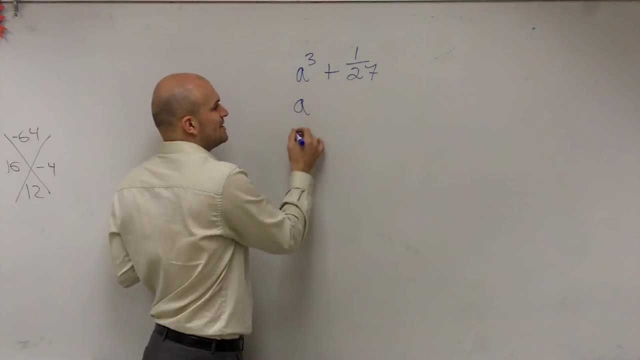 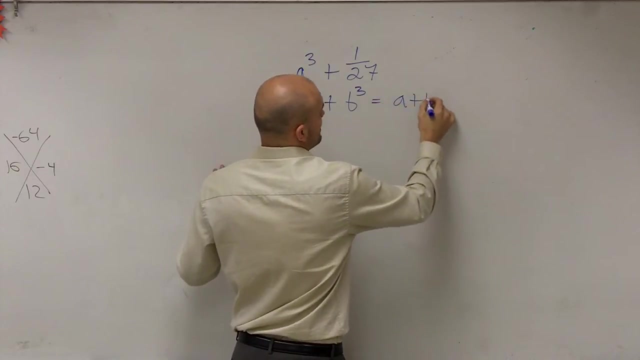 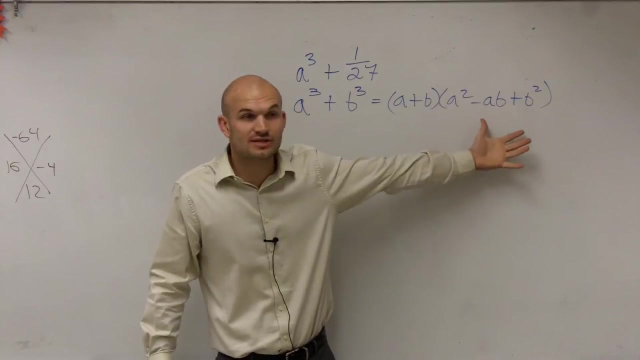 So if we're going to look at the sum of two cubes, that means we're going to have 8 cubed plus b cubed, And that can be written as a plus b times a squared, minus a times b plus b squared. So rather than doing the factoring and all that kind of stuff, if we can figure out what a and b are, we can simply just plug it into this formula And that's the factored form. That's what the factored form looks like. 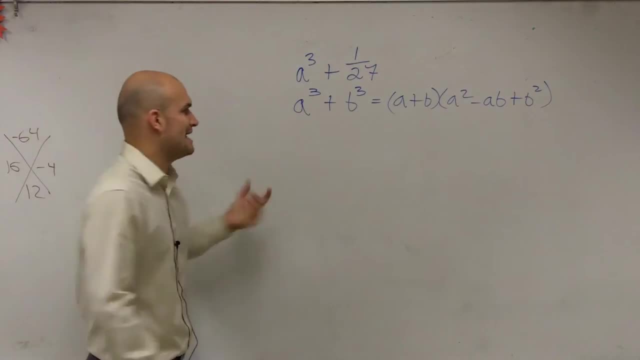 So what we need to do then, ladies and gentlemen, is we need to determine what a and b are. So what we say is: can we write this term and this term as factored terms, So you could say a cubed. So a cubed, doesn't matter what the variable is, is going to equal this one, which is a cubed. Then our b cubed is our second term, which is equal to 1 over 27.. All right, So if a cubed, right, we don't need to just figure out what a cubed is, We need to figure out what a is. 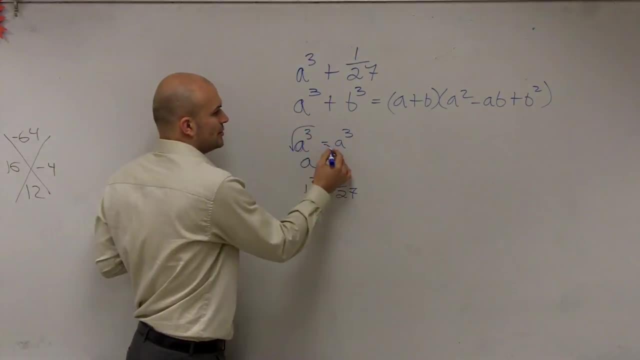 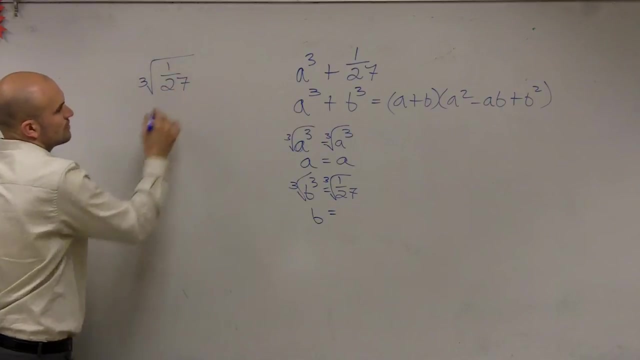 So if I have a cubed, then what's a? Well, to do that, you take the square root, or, sorry, the cube root of both sides, and the cube root of a cubed is just a, Then what I need to do over here is take the cube root of b, because I need to figure out what b is as well. So the cube root of b is going to provide me with b, and then the cube root of 1 over 27.. Correct, How do we do that? All right, Well, remember, ladies and gentlemen, with square roots.